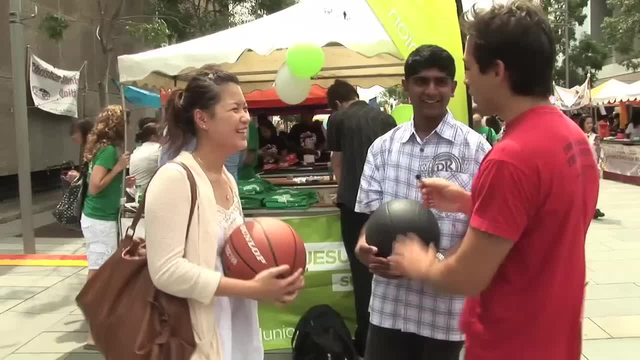 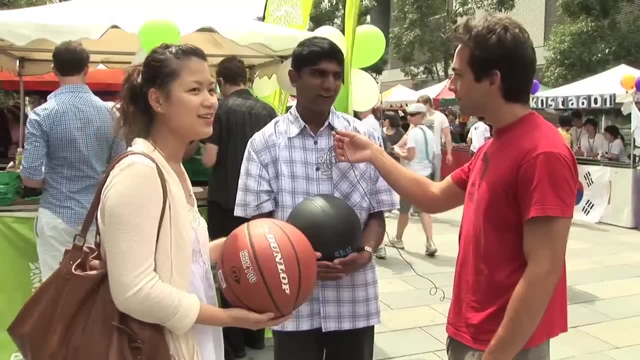 so they reasoned that the force on them must be the same. Tell me about how the gravitational force on this ball compares to the gravitational force on that ball. The force is the same. It's going to be very similar In terms of gravitational pull. they're both at the same and they'll fall at the same rate. 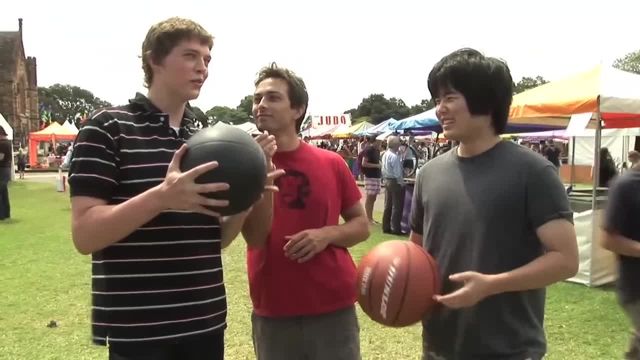 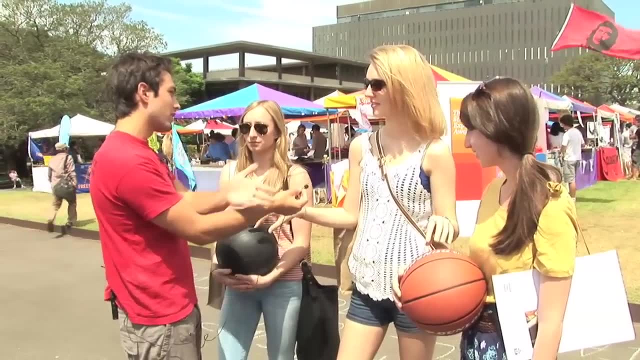 I'm not like Einstein. but same gravitational force around the whole world. right, Because the gravitational pull on the earth is the same on both objects. Are you saying that the force on them is the same? The pull is the same, But you felt the pull and you've told me the pull is different. 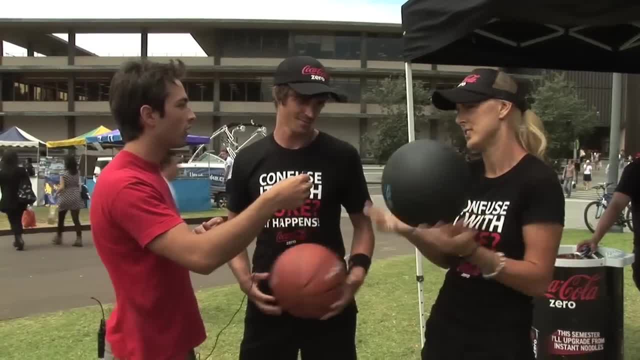 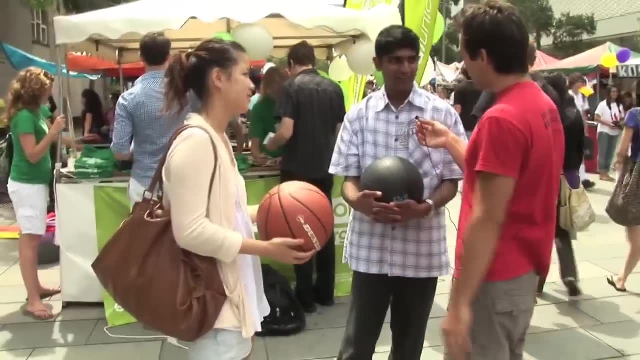 No, I said the weight is different. I didn't say the pull is the same. It is heavier and has more gravitational pull. but when I drop them then they get equal a gravitational pull somehow, Don't you think it's going to be like five times as much? 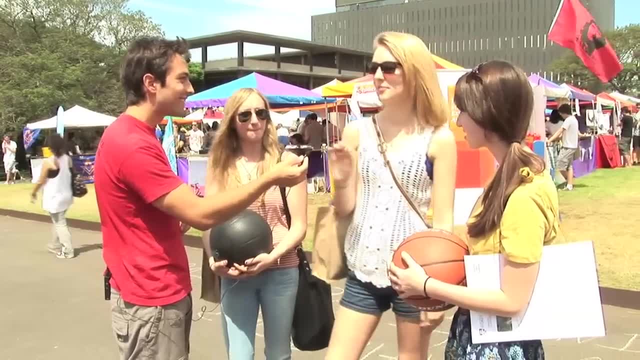 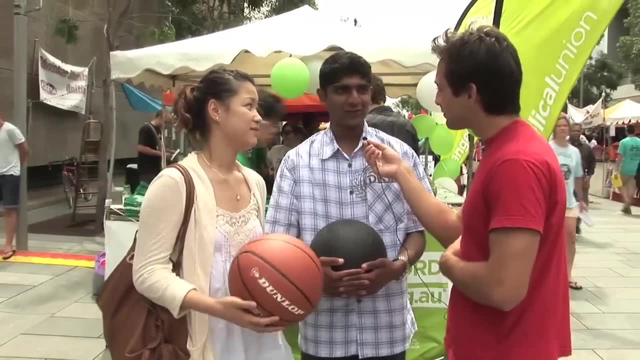 Yeah, you think, but it's not The way you're asking it. yes, but scientifically speaking, no. The gravitational force on both these balls are the same. Okay, The gravitational force on both of these balls is the same. Is that what you actually believe? 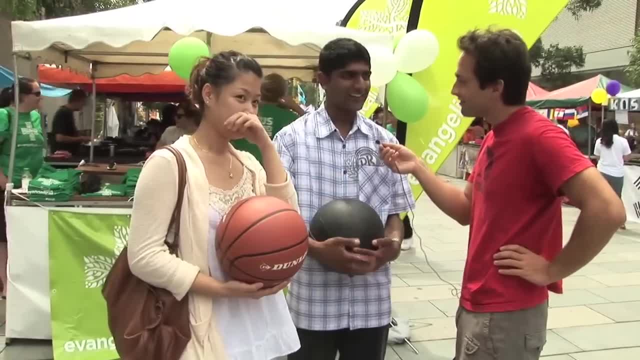 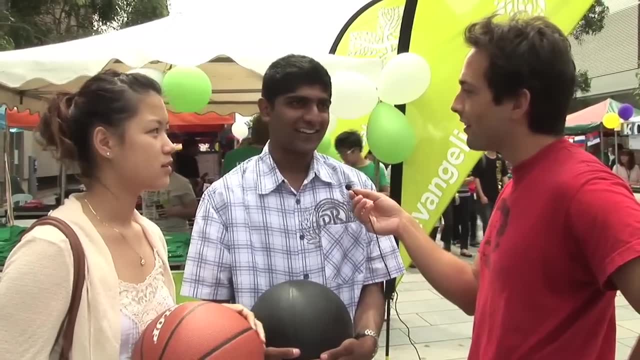 No, but it is. Tell me what you believe. I believe it should be more on this, simply for the fact that this is heavier, and just intuition tells me that it should be more. but after learning physics, we learned that it is actually the same. 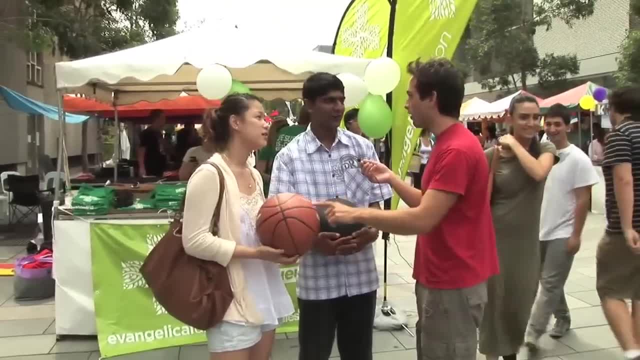 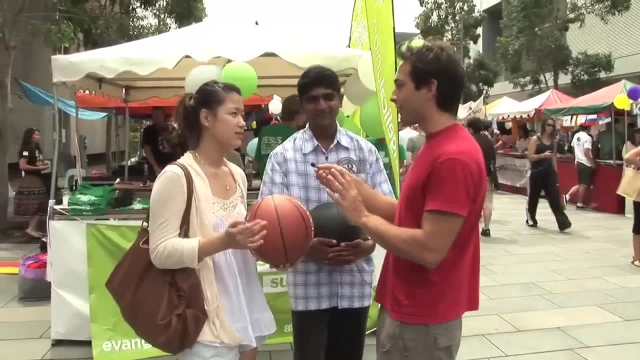 I actually think the force on this ball is more than the force on this ball. No, you don't, Just a little bit more. I swear, I am not trying to mess with you, So Like in real life, In real life and in physics, I will tell you that the force on this ball is more. 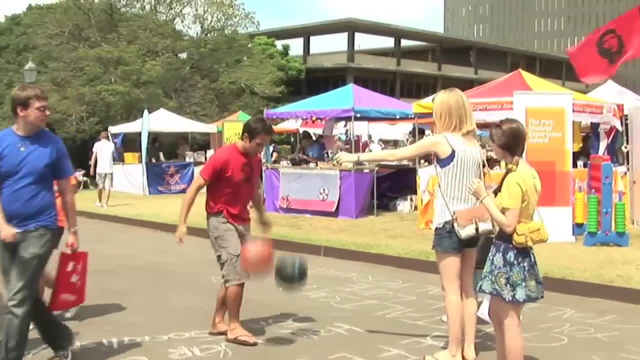 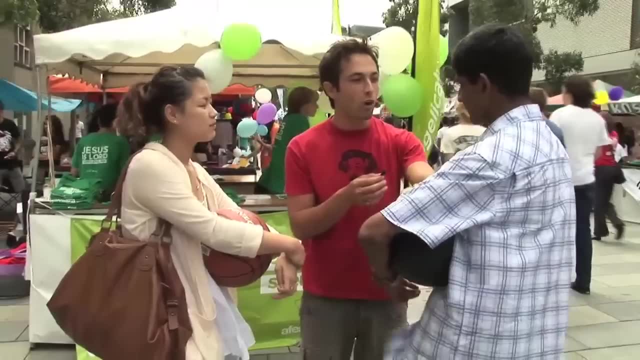 All right, Ready, Three, two, one, Yep, Yep See. Same time, Same time, Same time. The force on the medicine ball is like a lot more, because it has got a lot more weight, it has got a lot more mass, but it has got a lot more inertia. 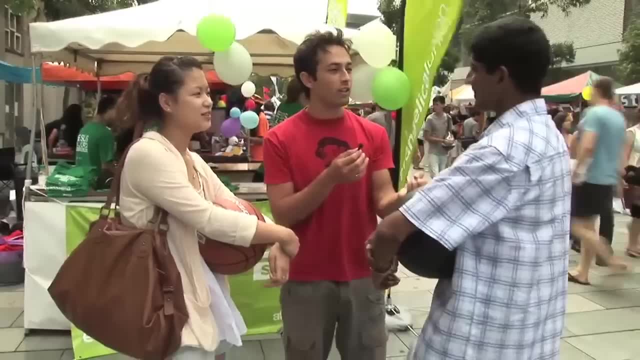 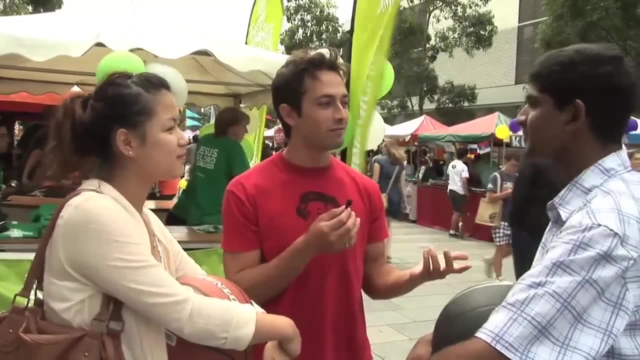 Yeah, yeah, Oh, You guys remember that right. It has got a lot of resistance to acceleration, so it takes more force to get it accelerating at the same rate as this ball, And that is why they accelerate at the same rate. 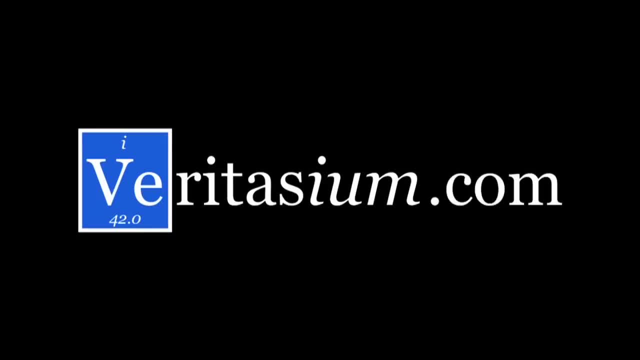 Thank you guys so much for playing along. Thank you, I appreciate that. Sorry, Jared, That is all right.